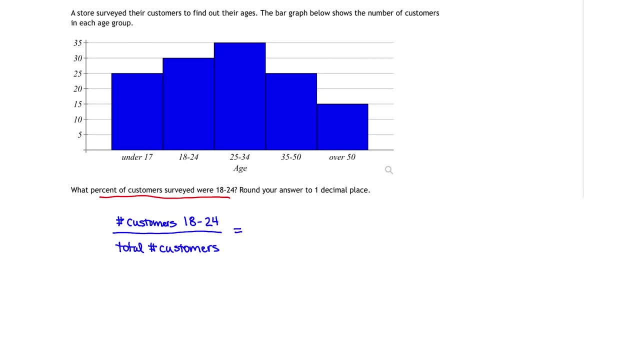 with the customers in the ages of 18 to 24?? Well, we look at our bar graph and we focus right there on the ages of 18 to 24.. If we look at the height of the bar graph and we read it off of the vertical, 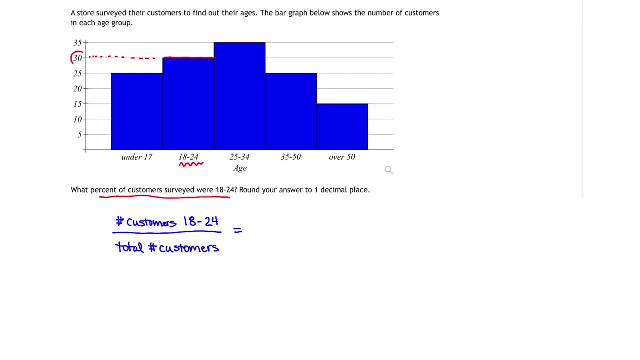 axis that's going to tell us how many customers fell in that age group. It looks to me like there are 30 customers that fell in the age group of 18 to 24 years, And so that means the number of customers 18 to 24 was actually 30. Now we need to divide by the total number of customers. 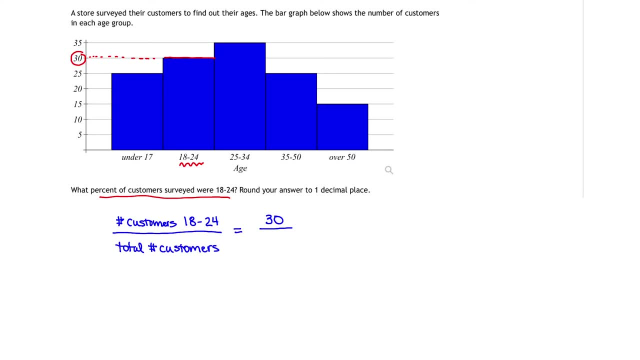 So we actually have to calculate the amounts for all the other age groups, From 18 to 24, we have 18 to 24. And so we have 18 to 24.. And so we have 18 to 24.. And so we have. 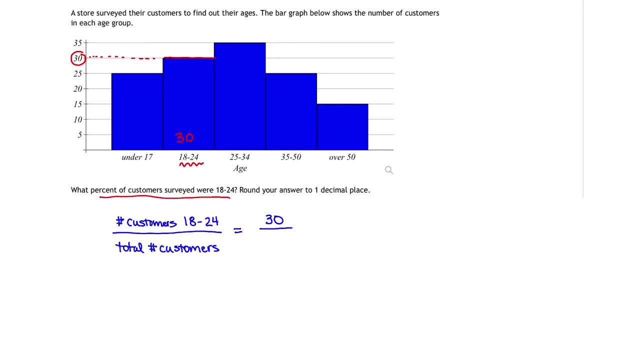 18 to 24,. I already know I have 30 people, So let's go and start getting the other values Under 17,. well, how tall is under 17?? Well, that corresponds to 25 people. looking at the vertical axis, 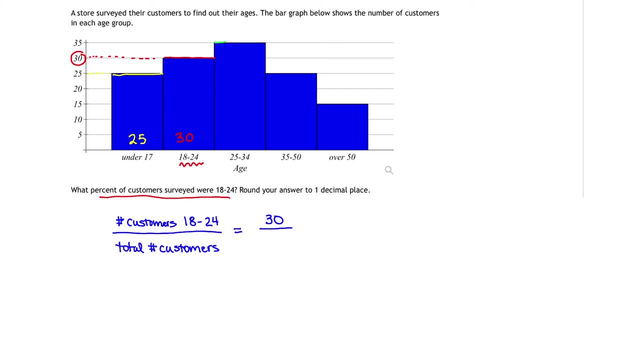 25 to 34 age group. that corresponds to 35 people looking at the vertical axis, Under 35 to 50,. 35 to 50 gives us, again looking at the vertical axis, 25 people And then going down we have over 50.. 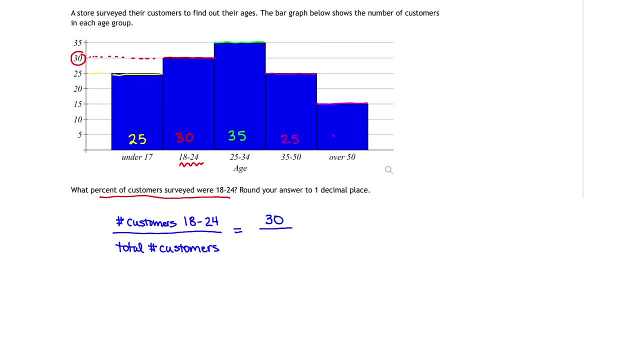 And the total number of people over 50 looks to be 15.. If we take our customers then to get the total number of people over 50, the total, what are we going to do? We're going to add all of those amounts. 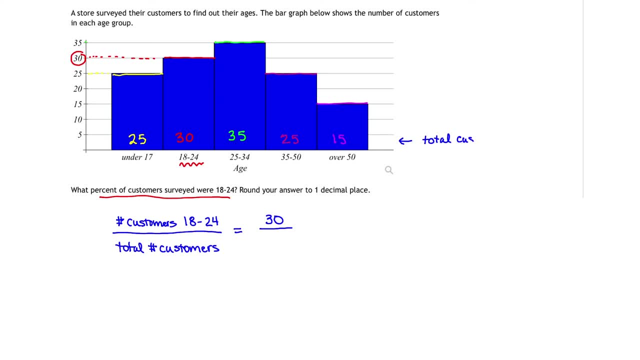 In other words, to calculate the total number of customers, we're simply going to add 25 plus 30 plus 35 plus 25 plus 15.. And that gives us a total of 130 customers altogether. That's the amount that we can divide by in order to get our percentage.